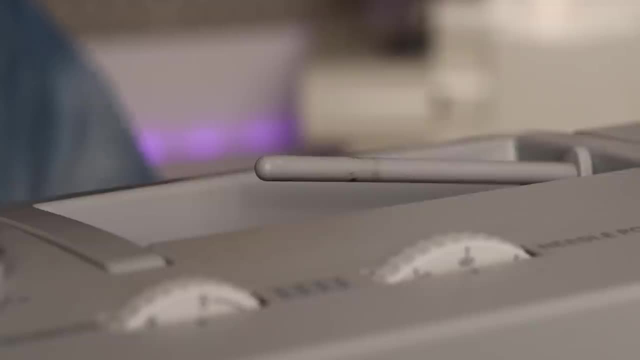 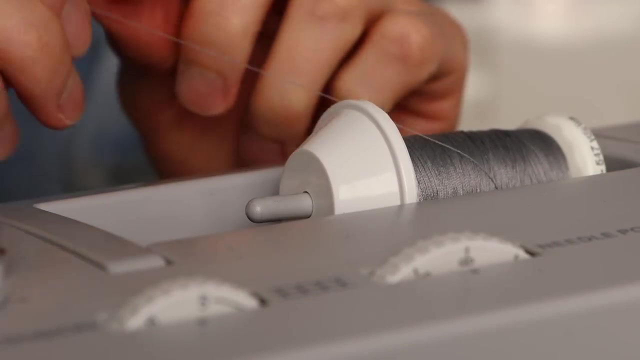 you should load up before your first time sewing. i start by putting my spool of thread on the spool pin and with the cap to hold it in place- remember the big side of the cone closest to the spool. then i find the fixtures to thread my machine specifically for loading the bobbin. the bobbin. 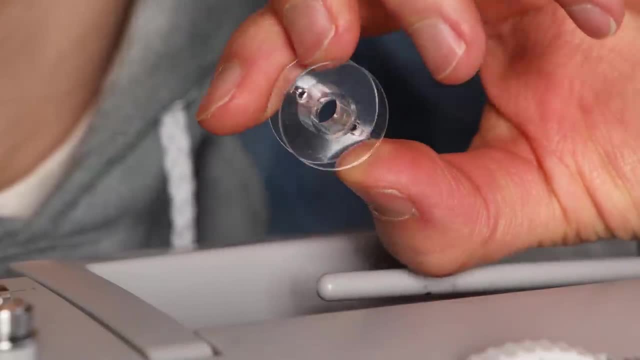 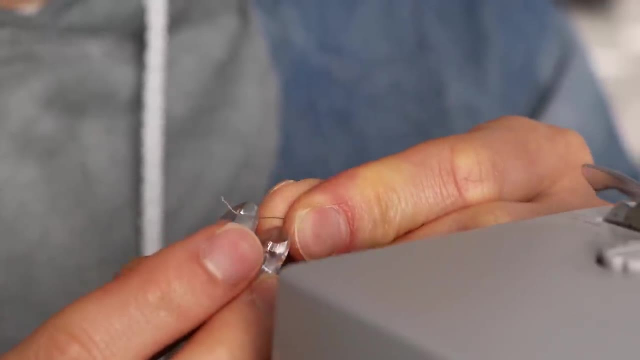 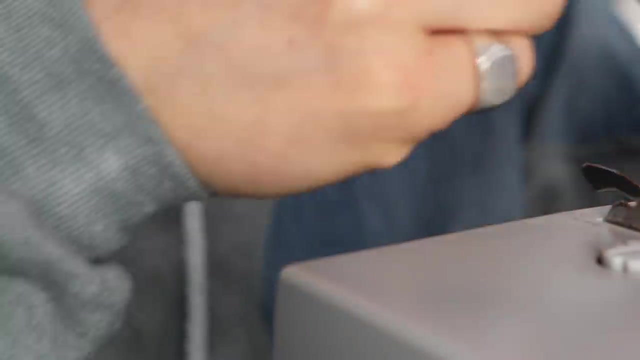 is this clear looking wheel and it typically has a hole on the wall to feed the thread through. once you have a bit in it, use your thumb to hold the thread as you manually wind five or six times to get the thread to hold on to the bobbin. then you load onto your machine. for mine, you push it to the. 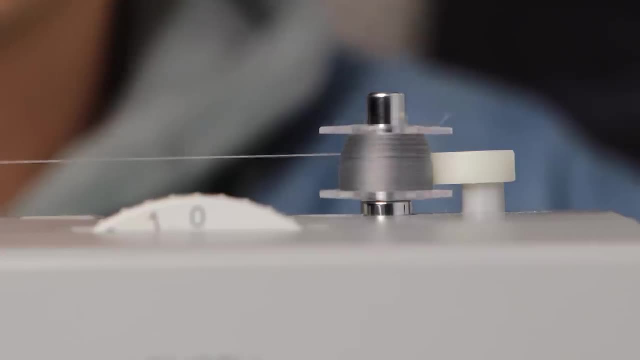 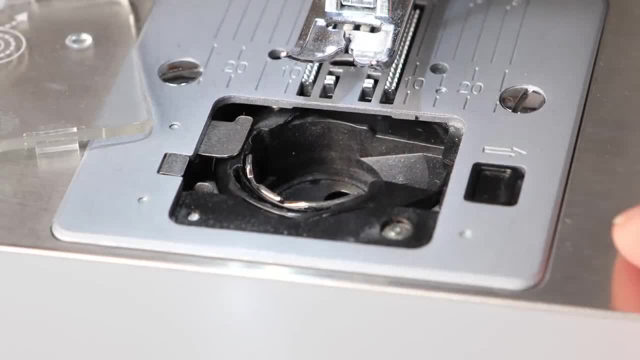 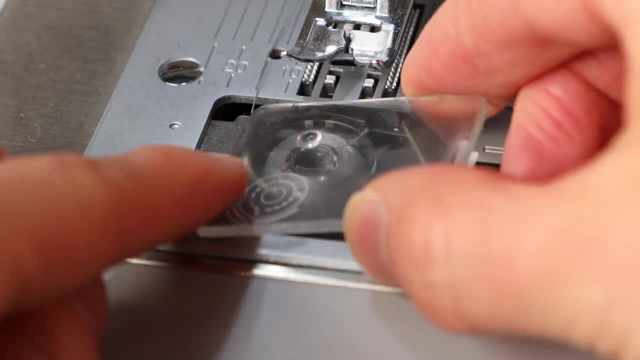 cover for the bobbins home. so you just got to unlock that, drop the bobbin in and there's some visuals on that covering as well. so use that visual as a guide for how to load the bobbin thread, and i usually leave the cover slightly cracked just for now to load the bobbin thread. 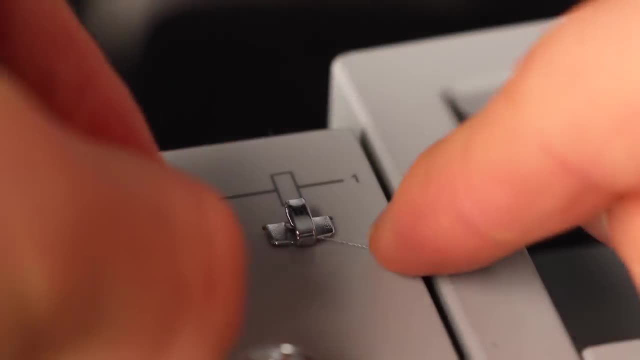 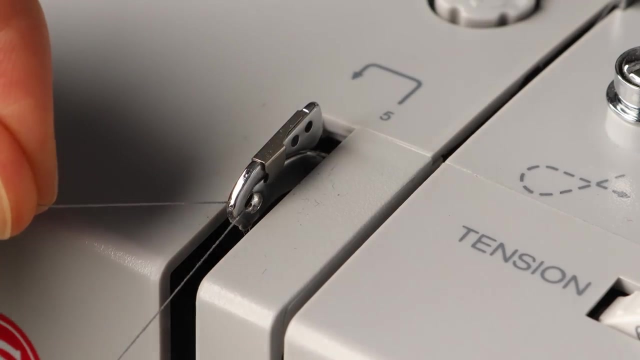 the sound company has made it real easy. so all you got to do, as long as you can count, is use your hand and, as you're counting, follow the thread through the hoops and fixtures so you could properly thread your machine. this is how i thread the singer 4423 and i think if you have a different 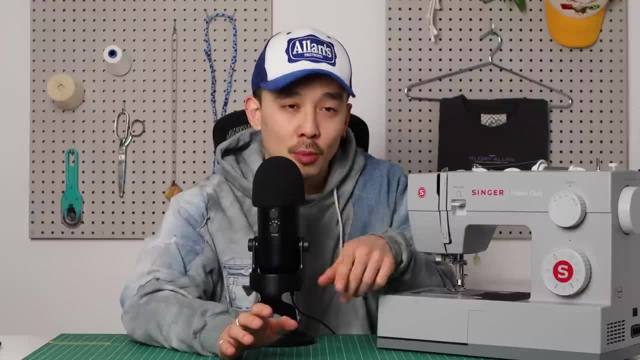 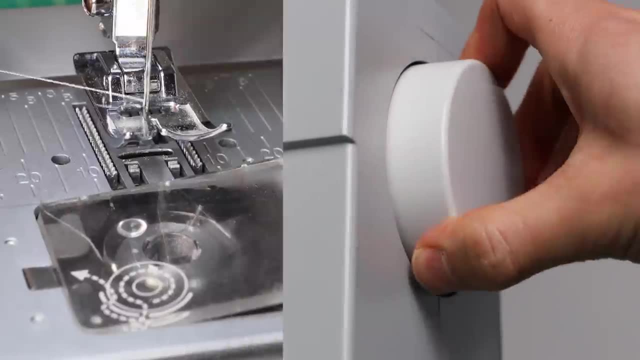 machine. it's going to be slightly different, but generally they fall somewhat of a similar path. once it's in the needle, use your left hand to hold the thread and use your right to pull the wheel towards you, which is counterclockwise, so that the needle goes through the bobbin thread. 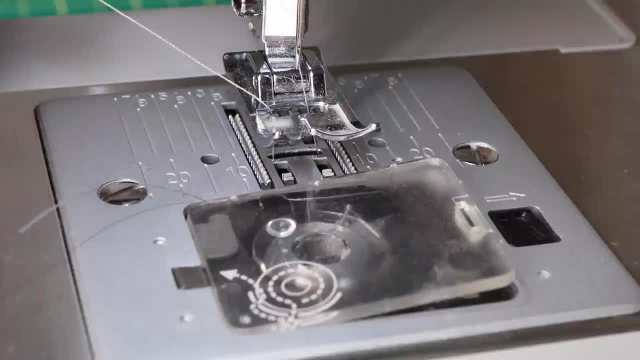 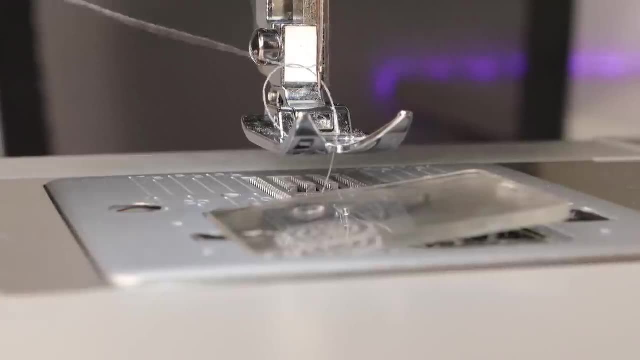 you can see through the clear cover that the thread will wind underneath and catch the bottom thread and bring it up to the surface. when it does, you let it pull the bobbin thread up and, once you see it, pull it through and place both threads underneath the presser foot. sometimes when the 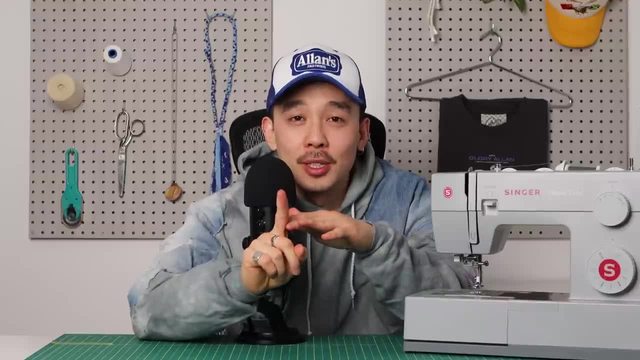 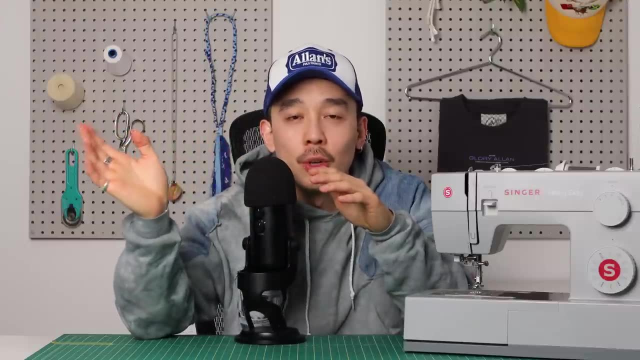 bobbin lid is closed. the bottom thread is locked into place so it can't be pulled. that's why i like to leave it a little bit cracked so that it's free to move around. make sure you have at least three or four inches and when you pull the bobbin thread you can see that the thread is. 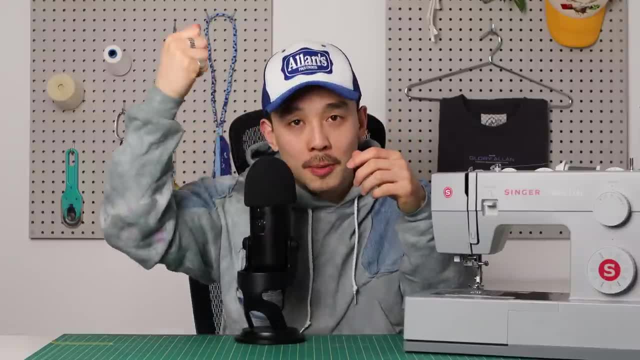 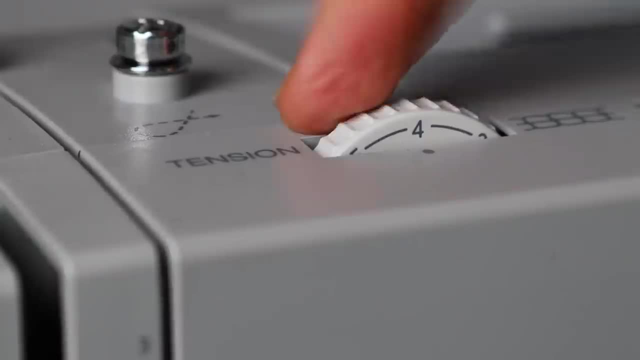 Ziploc to your right side of the machine and if you pull it to one side, this속 Abertox will route the thread. then the operator will move the bobbin toward you, the bottom thread will go underneath, scoop it up and pull it to the surface and then, now that it's all threaded, 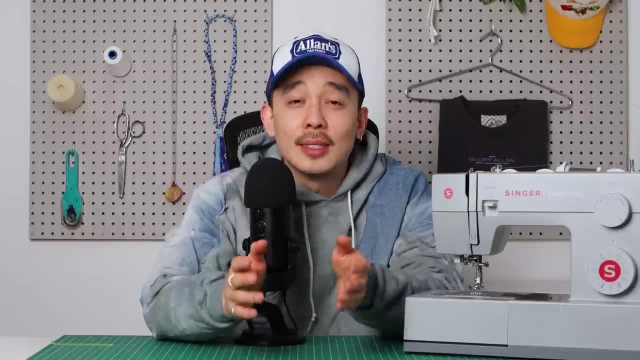 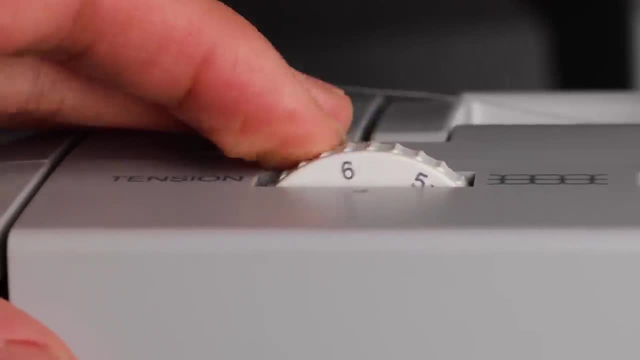 you can pop that cover back down. now let's talk about the tension and the stitch length. textbook definition: sewing tension is the amount of thread that passes through the machine to create each stitch. so the more thread that passes through, the looser the stitch is going to be, and the less thread that passes through, the tighter the stitch is going to be. 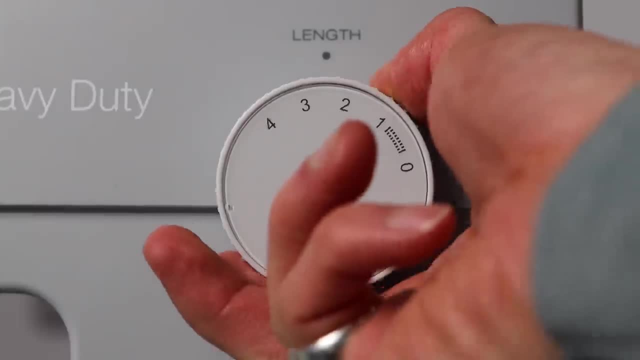 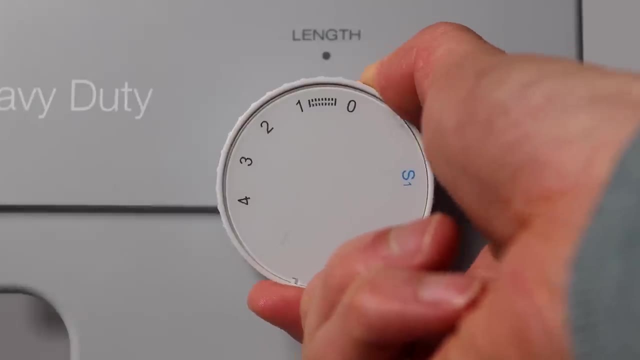 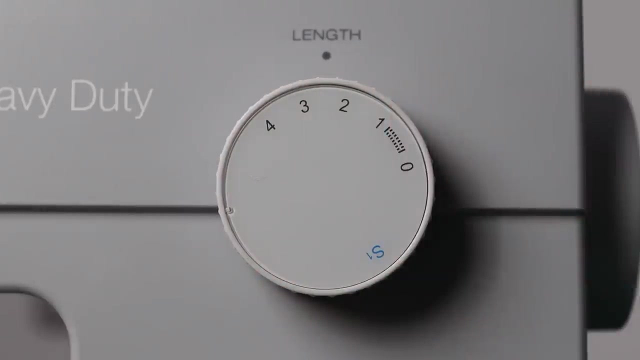 between two consecutive punches of a needle. the bigger the number, the bigger the stitches are gonna be. if you go into the lower numbers, I think below one is where you start getting it's like really tight for buttonholes. so usually just go between one and four and then four buttons less than one. on average you're. 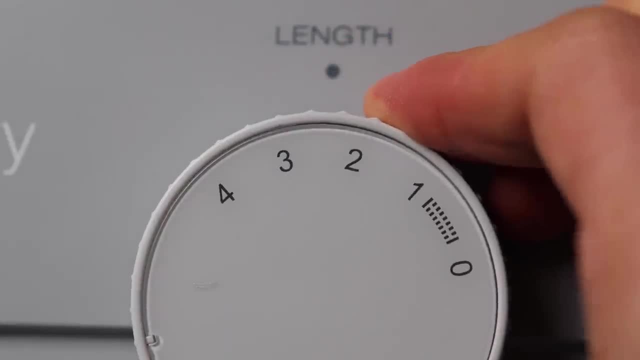 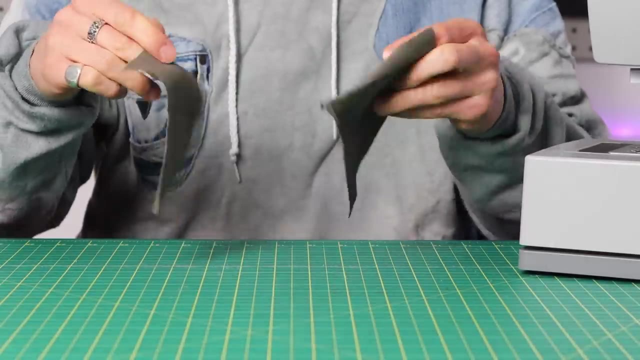 looking at a tension of four and a stitch length of 2.5 before starting any project. take that material, cut a test piece out, put two layers underneath here, because typically you're sewing two layers at a time, so you want to mimic the same thing you would do in the real project. what I'd suggest is start at 2.5. 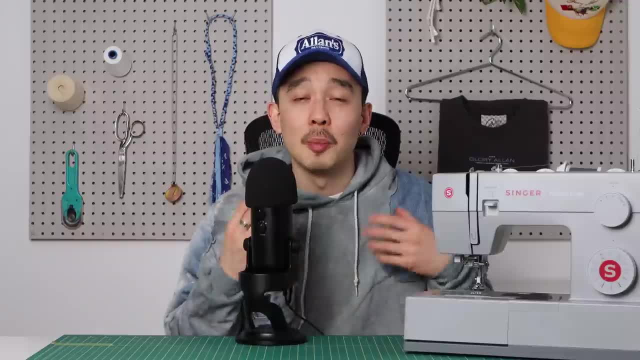 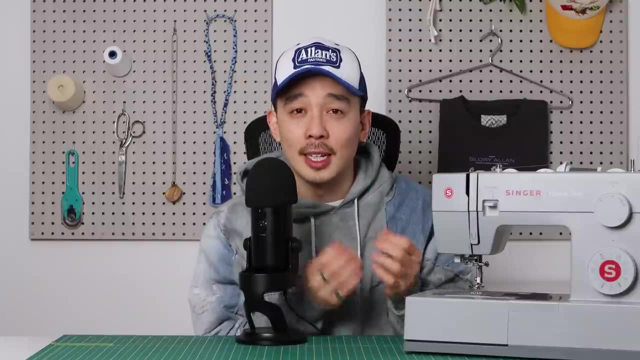 and 4, and you're just gonna adjust the tension and stitch length based on your intuition until the stitches come out even, meaning the bottom stitch and the top stitch look very balanced. that's when you're gonna know you have it right. these settings will vary depending on what fabric you're using, whether it's 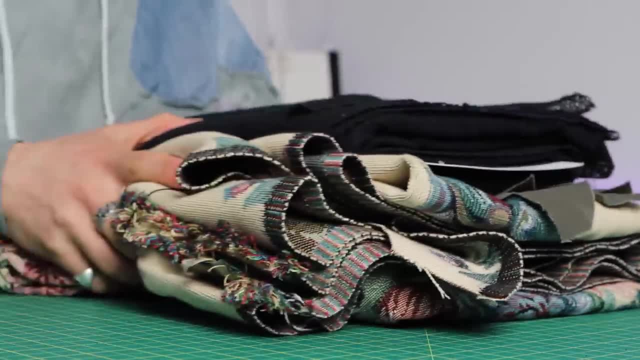 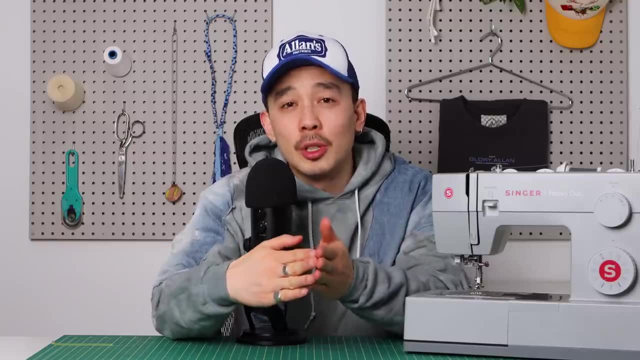 lightweight, midway heavyweight. generally you want to use a shorter stitch length for the lightweight material and then when you work with heavier weight materials like denim or canvas, that's when you want to go into a bit lengthier of a stitch length. the bobbin tension is already factory set, so just worry about the top dials now. 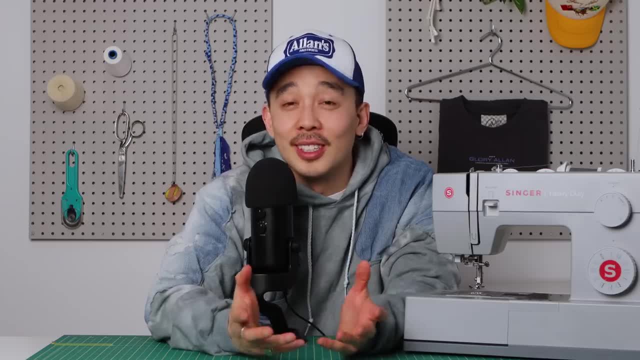 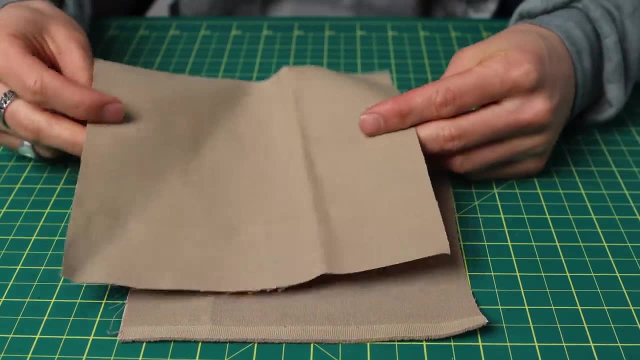 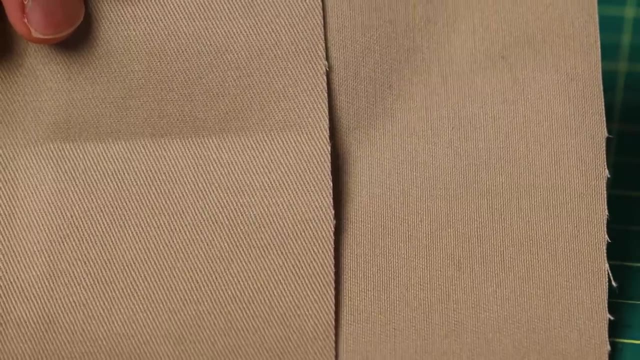 that the machine set up, it's time to learn the sewing basics, which is the exciting part. most fabrics- not all fabrics, but most- have a right and a wrong side, the right side is usually a bit better looking, the wrong side being more rough. if you look at this, this is cotton twill and if you look up close on 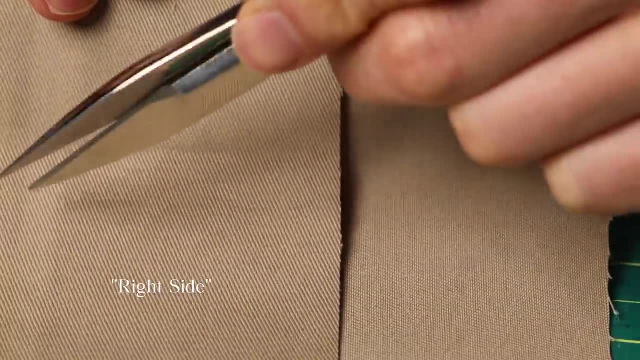 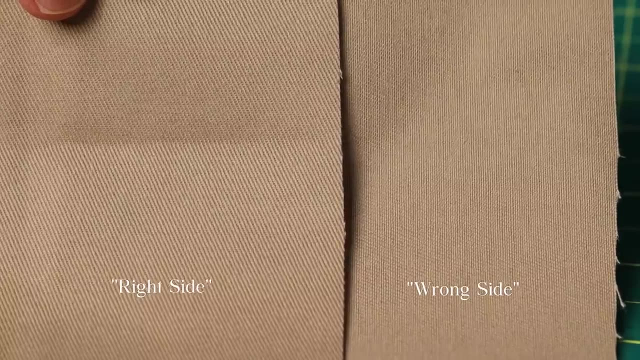 the left side you have these diagonal woven lines and then on the right side it's just very rough. if you have your material in front of you, examine it. you can see the difference. you could tell based on shine. sometimes you can tell based on feel, on looks. use your. 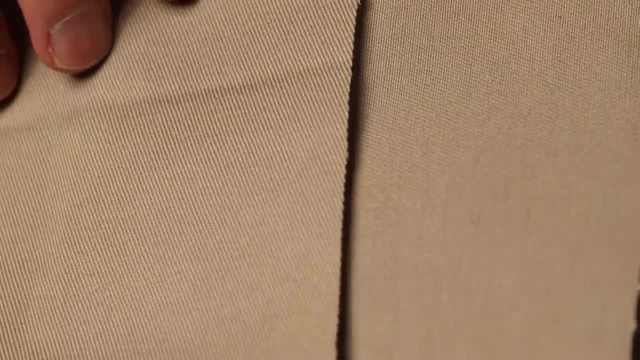 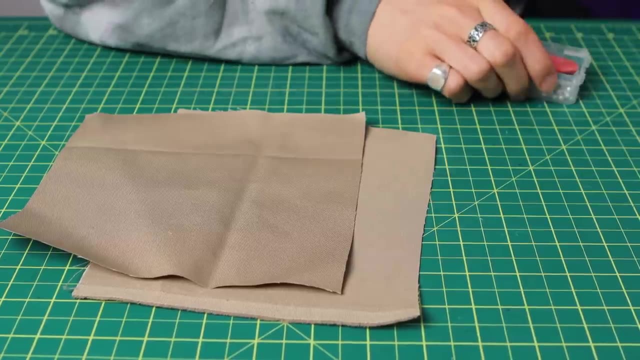 intuition and try to figure out which is the right and wrong side. now, when you're sewing these panels together, you typically want right sides facing each other, and then that means wrong sides are on the outside. so I'm going to illustrate this by putting a chalk X on the middle of it, so the fact that you recognize the candle you're not going to cut, and then you're just going to leave it the way you always 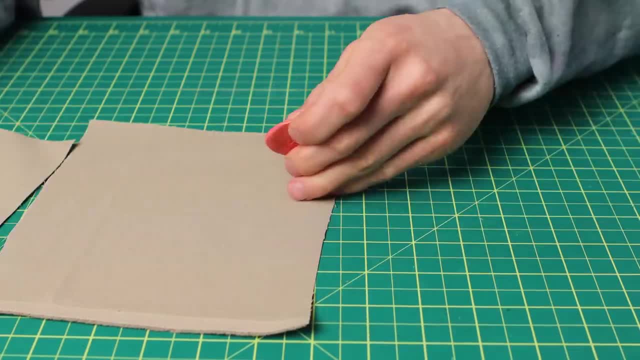 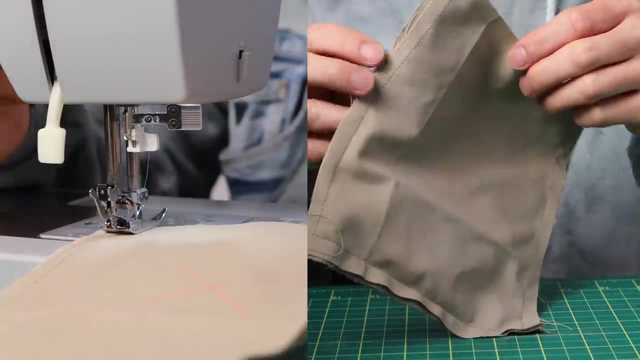 were before making calculations on which side will really stick to each other, be the wrong side of both these fabrics, and if I want to sew them together I want the X's on the outside, meaning right sides are facing each other, so that once I'm done sewing and I pull that. 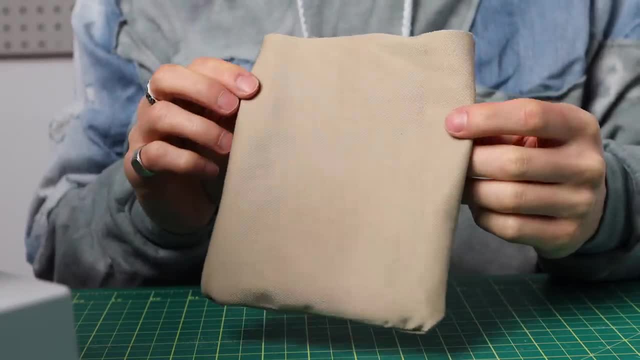 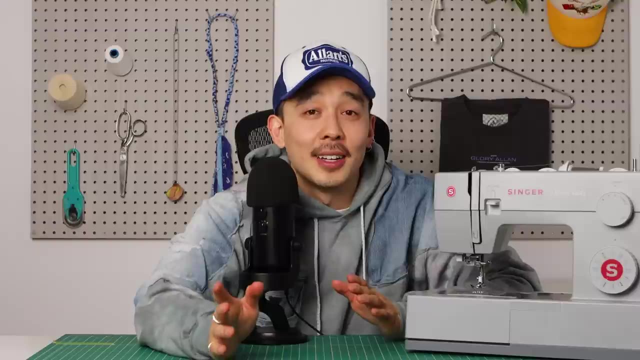 inside out. now I have the shape of the, the project that I'm working on, and I have the right side, which is the more polished finish side on the outside Side. note, if you want more advice and insights on sewing or you want to stay updated on the latest DIY kit free sewing pattern, that I drop 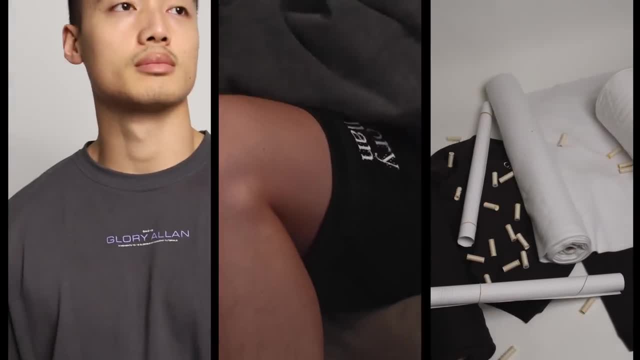 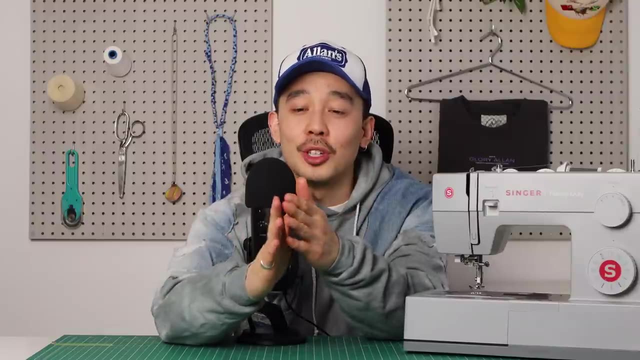 on my channel, subscribe so you can stay tuned to the latest. and then you have what they call a back stitch, and back stitch is how you lock in the stitches and it's usually what you do at the beginning and the end of every stitch. Let's say, we're going to sew along this blue line you want. 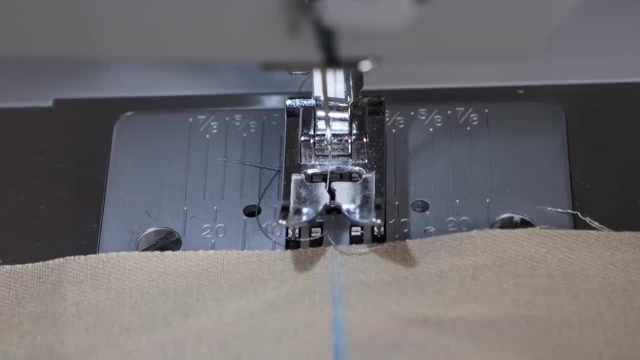 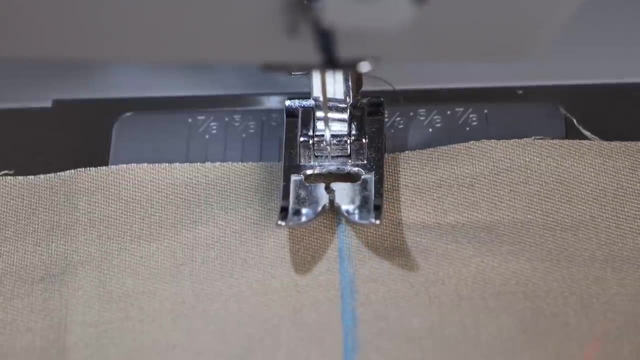 to put your fabric underneath the presser foot and you want to line up the fabric so that the blue line, which is the line you want to sew, is lined up with the needle not too far to the left, not too far to the right, and if you imagine the needle coming down, you want to make sure that the 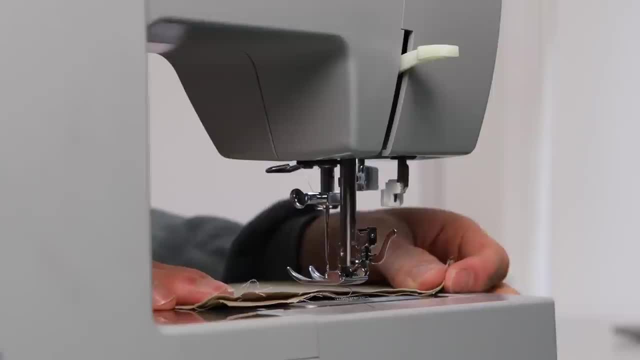 fabric is aligned with the needle, not too far to the left, not too far to the right. and if you is in enough that the needle will be past the edge of the fabric, Put the press foot down so that it holds the fabric. I usually do three stitches. 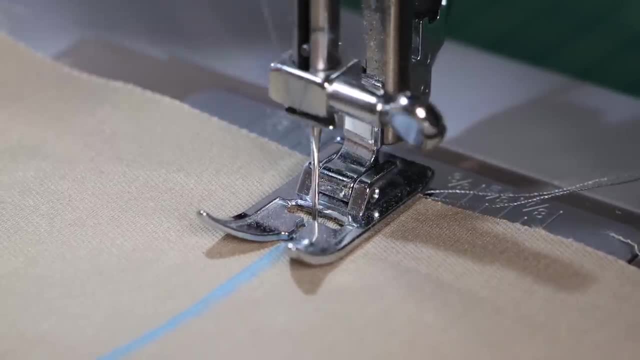 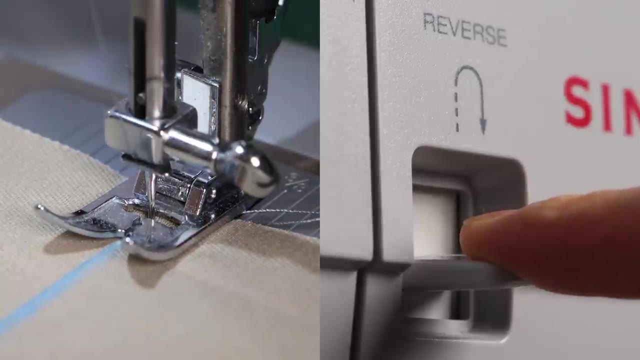 forward and then three stitches back. For my machine there's a lever that you pull down, and when you pull down you hold it and then use your foot on the pedal and that'll bring the stitches in reverse. What this does is it allows you to go. 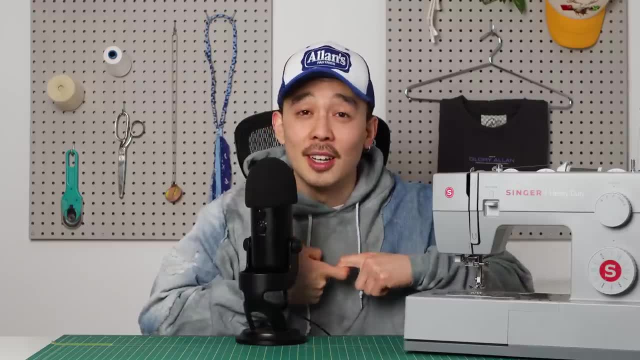 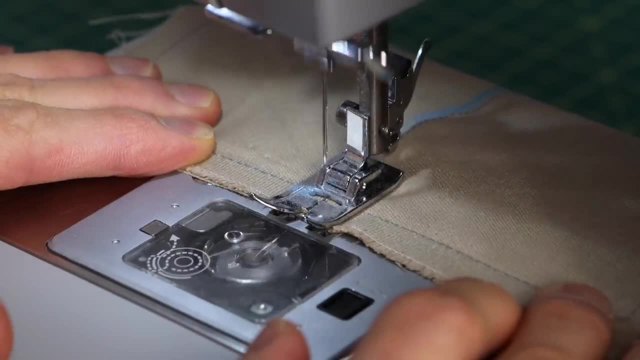 back over stitches you previously made so that it locks it in and there's less chance of your project unraveling. You'll run the same exercise when you get to the end. Sew near the edge, go backwards three stitches, forward three and you're done. Now let's talk about how you hold the fabric as you're sewing. I 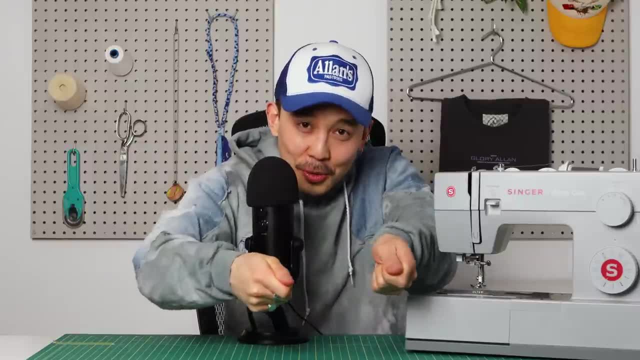 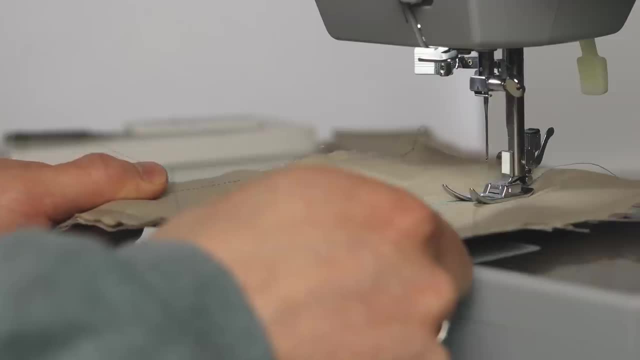 feel like there's not enough videos with advice on, like how to hold the fabric as it's getting fed in, so let's talk about it. Hold the fabric taut enough that you can control the direction. that way, you could sew in a straight line, or 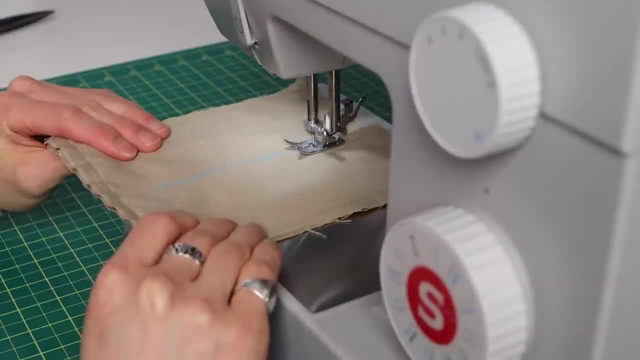 pull it and turn it the way you want, but don't pull too much that you're fighting the feed dogs, Because if you don't pull too much, you're going to end up with a lot of stitches and you'll probably get uneven stitches. I feel like everyone has their. 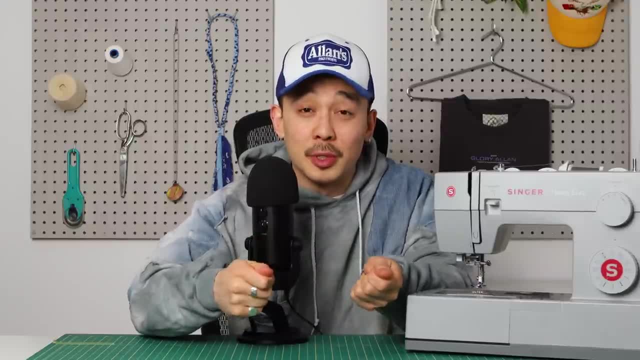 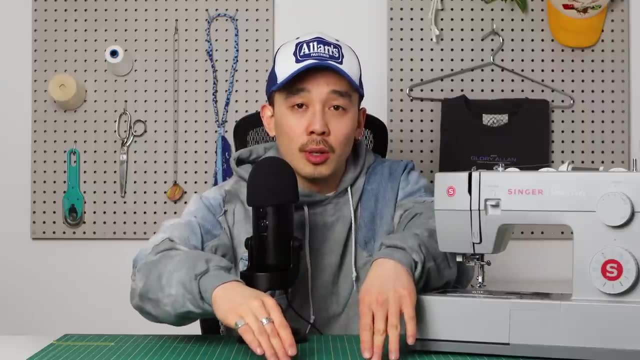 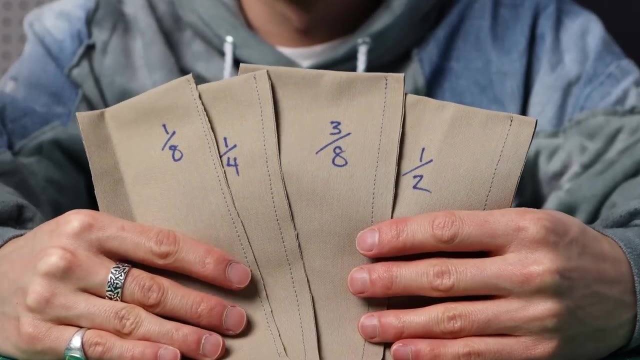 own way of holding the material. Sometimes you want to like grip it from the sides and pull. Sometimes you just want to be on top and apply pressure and pull a little bit, but I think generally a little bit of pull. however you hold, it is going to give you the control of the fabric. Now for the seam allowance. This 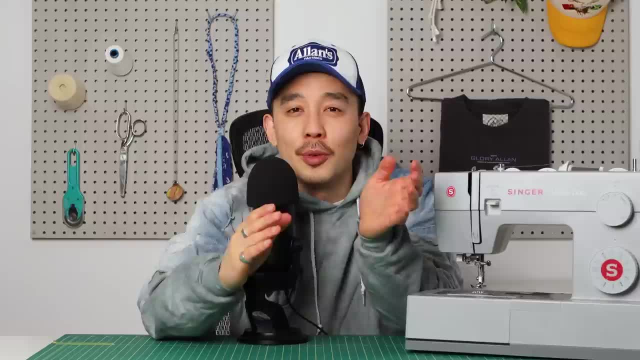 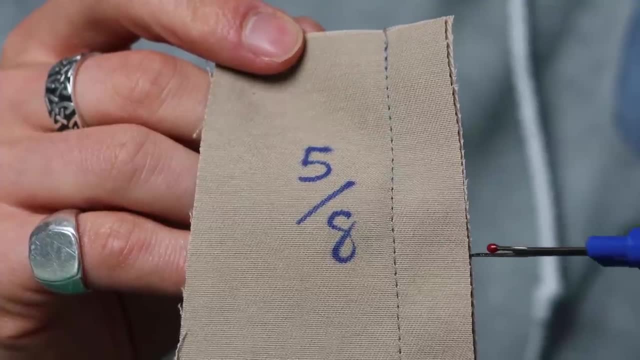 is like that mysterious thing. you hear about it and you don't really know what it is until it's time to learn about it. It is the area between the stitch and the raw edge of the fabric. Basically, if you're sewing, you can't sew right on the edge, because then the thread will have nothing to. 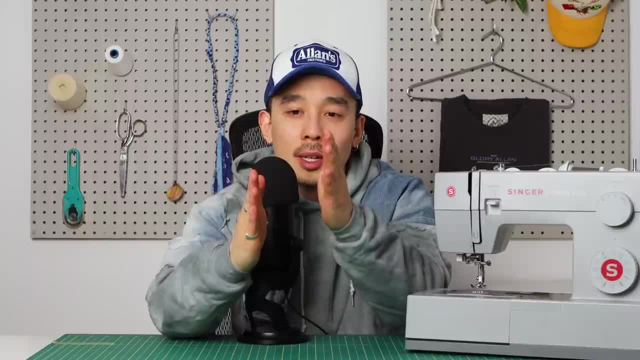 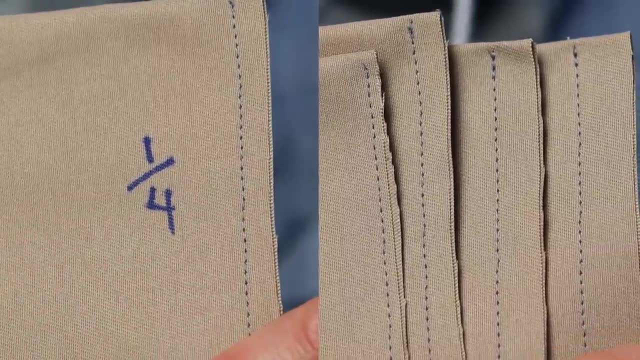 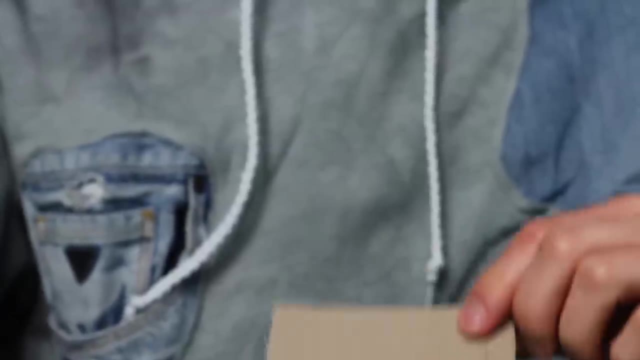 hold on to. so you have to go into the edge of the fabric a little bit and sew. Generally you don't see an eighth of an inch or quarter inch seam allowance, but I did it here just to illustrate the difference. as you increase the seam allowance, you increase the distance from the edge of the stitch For the most part. 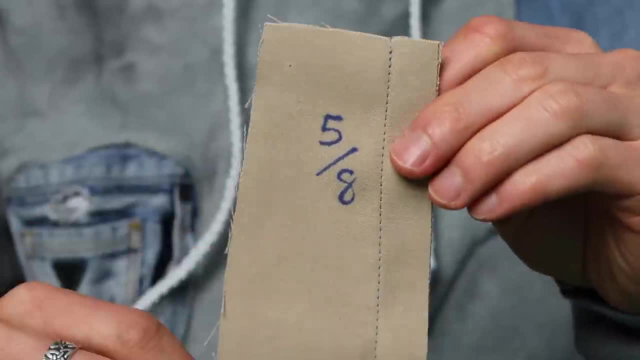 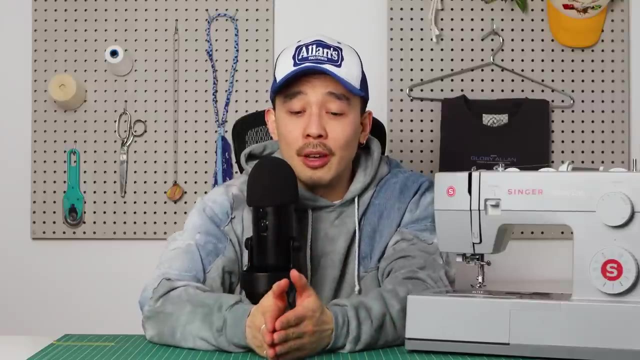 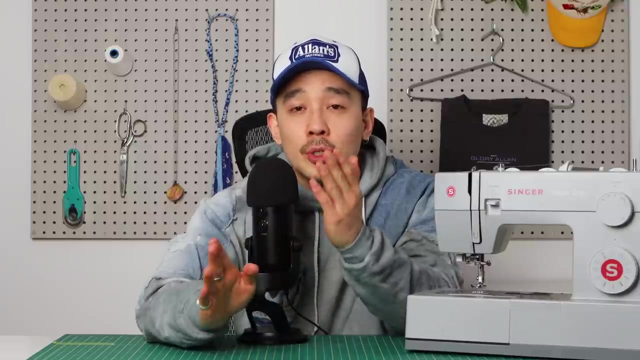 you'll see three eighths of an inch seam allowance, a half an inch seam allowance. Sometimes for trousers or pants they'll have a very, very large seam allowance and that allows tailors to take it apart and have a little bit more room to expand. 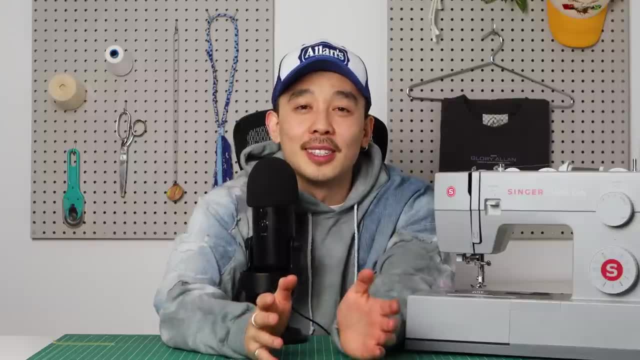 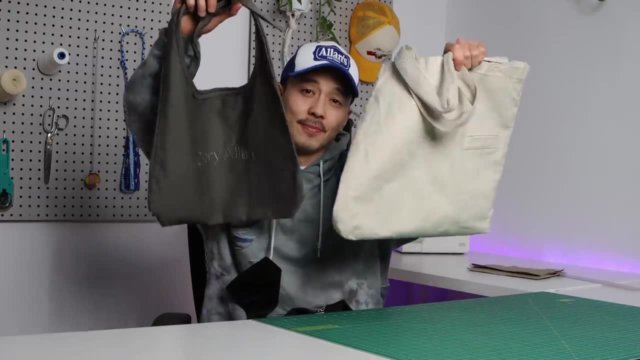 the fabric. if you need expanding Once you understand the basics, there's a playlist of sewing tutorials and projects on my channel that you can check out. There's beginner ones- I usually recommend the tote bag or the suna bag- but there's also some challenging ones for a little bit more. 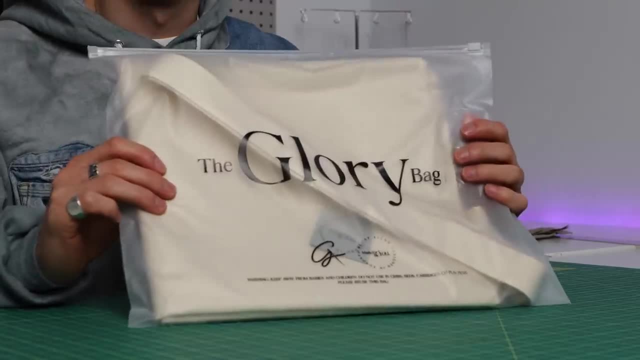 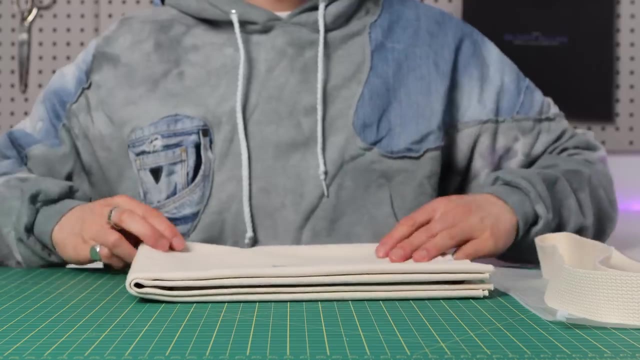 experience sewists, and all the projects come with a DIY kit, which is like a sewing kit that comes with all the fabrics, supplies, materials that you need for that sewing project. The tutorials are made for beginners, so even if you're brand new to sewing, I go step by step explain everything, so it's very 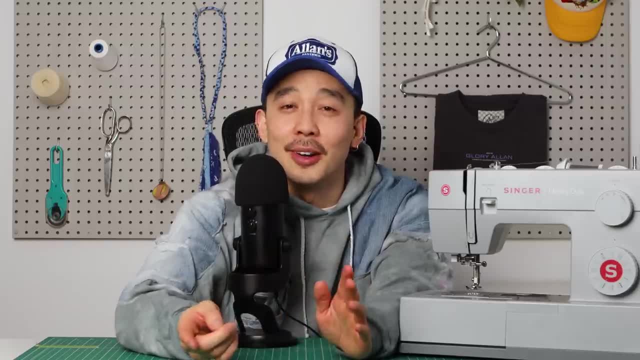 simple. So if you feel like sewing, check out the channel. if you feel like you want a DIY kit, check out my website. and until next time, peace.